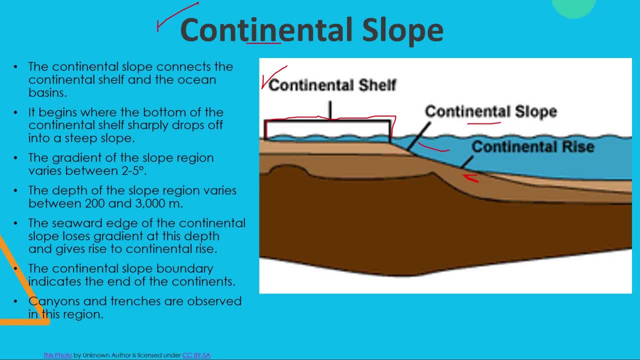 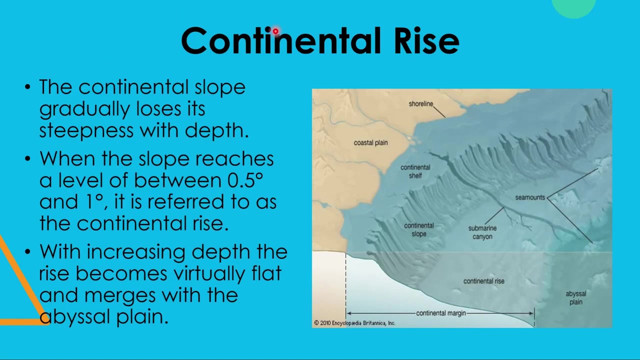 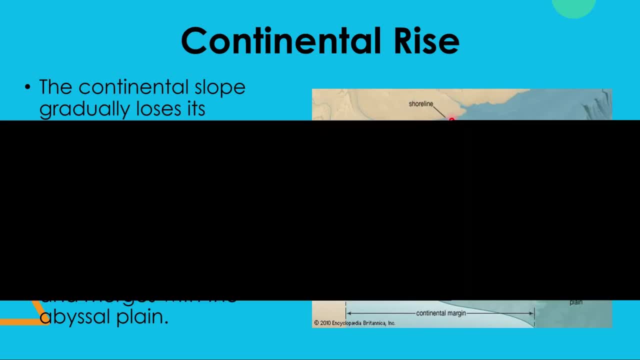 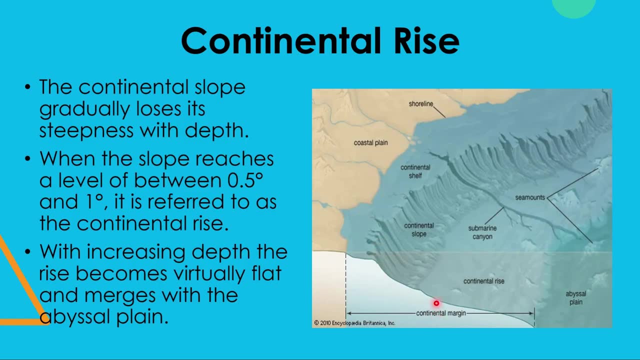 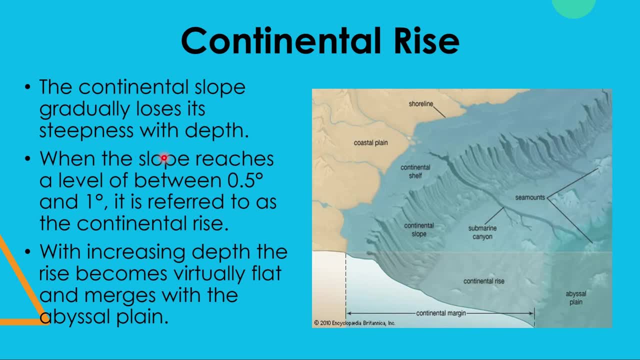 You are standing on the beach. you will move forward from the beach. you will get a slopey region. What happened by getting a slopey region? The depth of the sea increased. Now what will happen after some time, the depth is going to increase more. 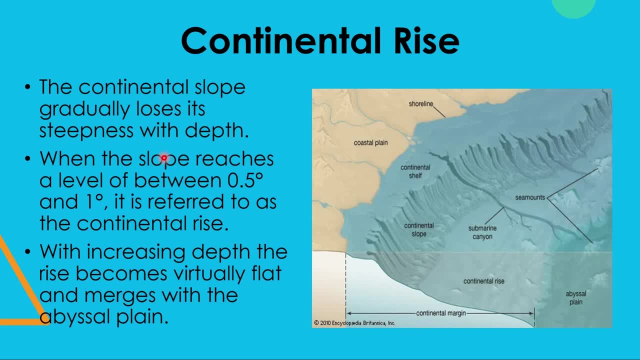 So as the depth increases, the steepness is automatically decreasing. So when the slope reaches a level of level between 0.5 to 1 degree, it is referred to as the continental rise. Look at this diagram carefully. The gradient here will be 0.5 to 1 degree, whereas the gradient of this region is more than that. 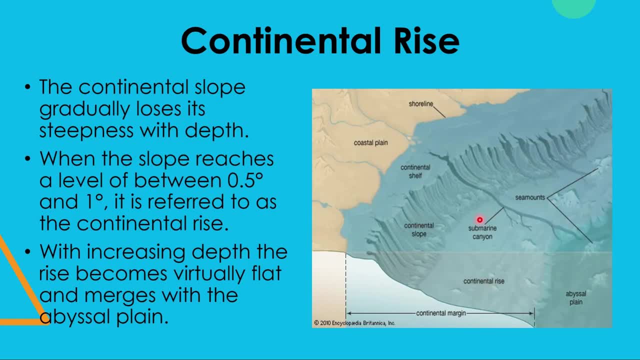 It is 1 degree to 5 degree, But the gradient of this region is 0.5 to 1 degree. So our continental rise, its gradient, is between 1 degree and 0.5 degree. As the depth increases, our ocean will become virtually flat and then it will merge with the abyssal plain. 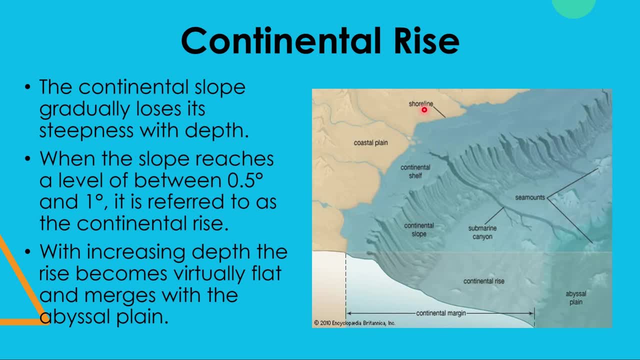 Meaning, first of all, what happened to the coastal plain. In front of the coastal plain, the continental shelf in front of the continental shelf, you went to the continental slope. From the continental slope, the continental rise, and after the continental rise, the abyssal plain came. 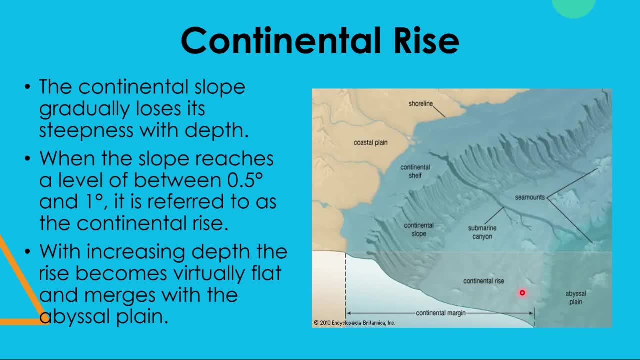 The abyssal plain is the region where everything is flat, right. How do the plains exist? So, without any height, without any slope, without any problem, you get a plain region. Okay, If someone asks where are the canyons of the submarine and where are the seamounts, 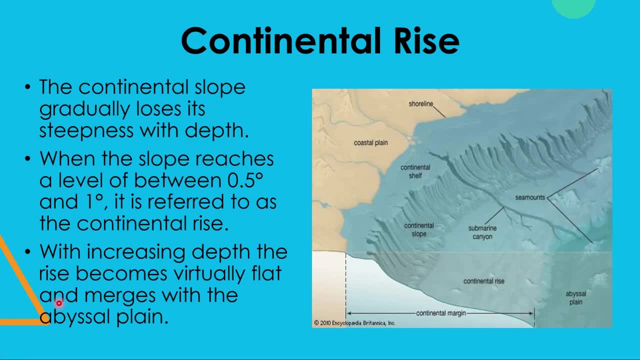 Seamounts are also present in the continental rise and also in the abyssal plain. Okay, If there is any confusion about this thing, then always keep this diagram in mind, That the seamounts are also present in the continental rise. Okay, 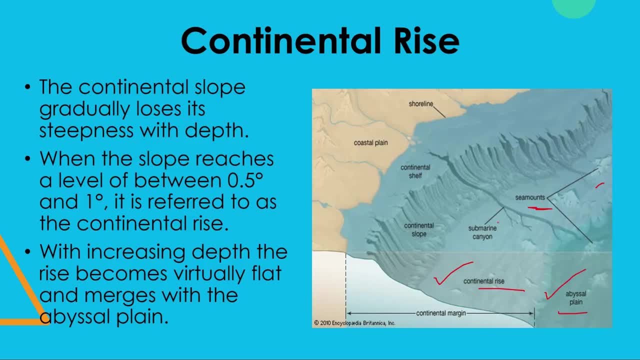 Okay, Okay, The seamounts are also present in the continental rise and also in the abyssal plain, But when you talk about the canyons or the trenches, they are only available at the continental rise. Right, If you go to the abyssal plain, you will not find trenches. 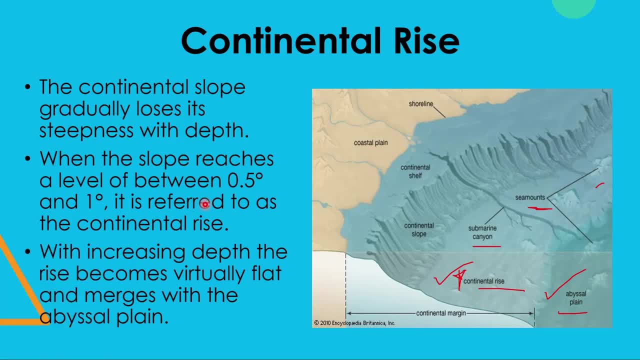 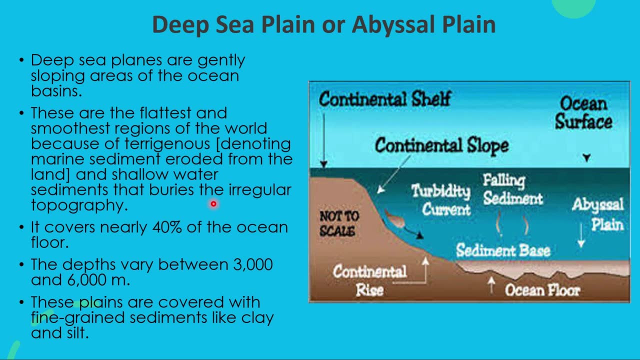 If you go to the abyssal plain, you will never find canyons. Okay, You have to keep this in mind. Then what happens to the deep sea plain and the abyssal plain Now? we said that we should start moving forward in the depth of the sea. 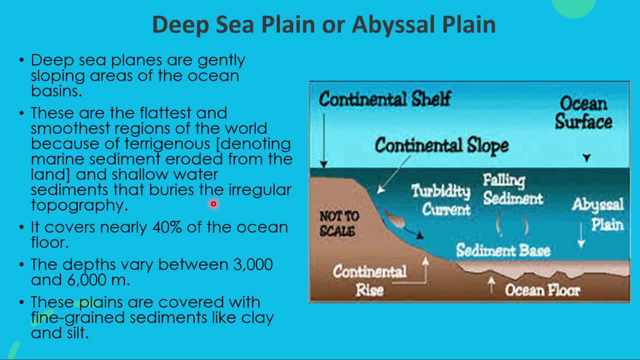 So if the continental shelf is flat, then we will not find canyons. Then theρο walk until it reaches the slope, then it rises up to the ocean floor. So our feel you then Okay, You have to fall into the Corporation Floor. 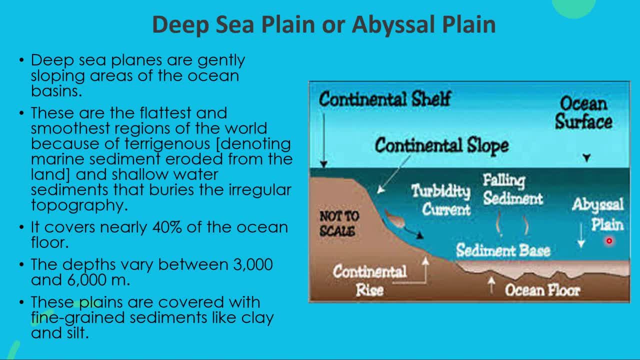 So you come into this portion of the Ocean Floor. The name of this portion is the abyssal plain, Which means that our deepest part of the ocean is claimed as the abyssal plain. What is its second name? It is also called the Deep Sea plain. 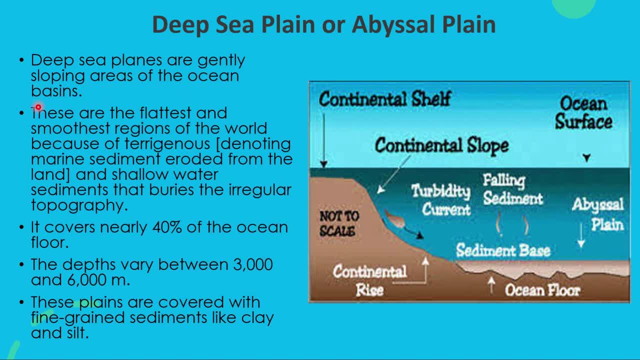 Okay, It means these are generally sloping areas of the ocean basins. Okay, It means that these are the flattest and the smoothest regions of the world- of the world because of the terigenius, denoting the marine sediments eroded from the land terigenius. 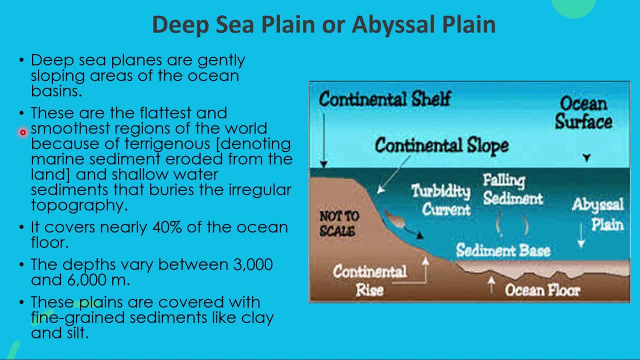 sediments. i told you that such marine sediments, which are eroded from the land, they come here and are deposited. okay, so here it starts to grow, due to which this region is considered to be a plain region, but the topography here is irregular. okay, plain in the sense that if you go to see height, 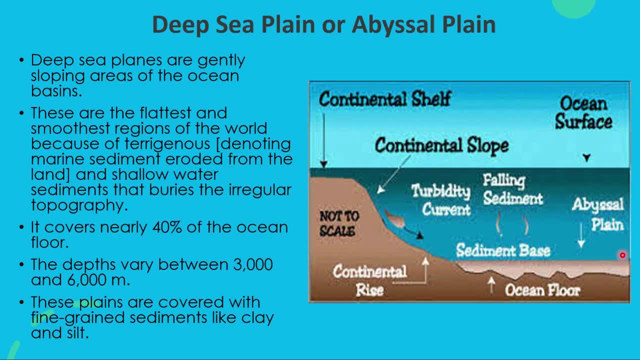 wise, then it is at the lowest height. it has a lot of depth from the level of the ocean, but topography is irregular. okay, then it covers nearly 40% of the ocean floor. now. its depth is 3000 to 6000 meters. now guess where the continental shelf was at 200 meters. 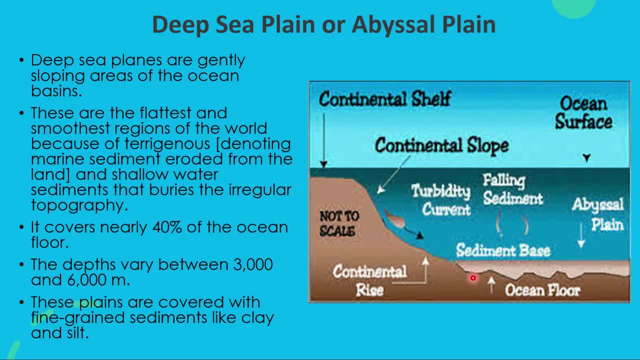 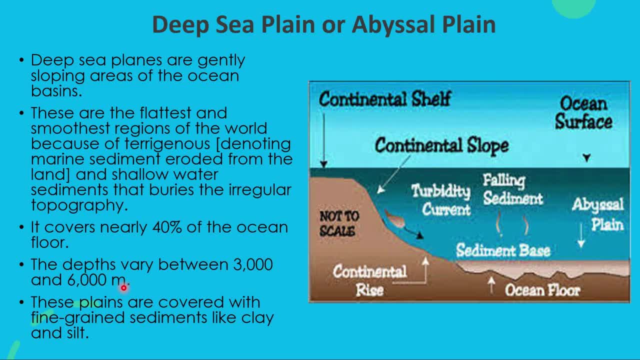 think: how much difference is there right? second, uh, the point is that these planes are covered with the fine-grained sediments like clay and silt. if the people who are under water, river rafting under water, who go to see, there are activities, there are sports, so you get to see this thing. 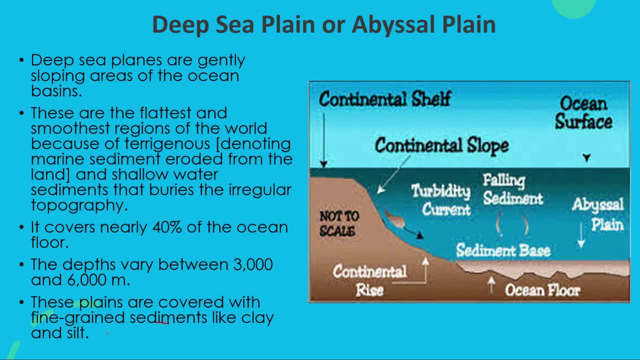 that when it is observed right. so here the sediments are fine-grained, so because of this planes, here a clay or a silt like structure is spread all over. okay, so these are the abyssal planes in which, these are the deep sea planes, in which the gently sloping areas of the ocean 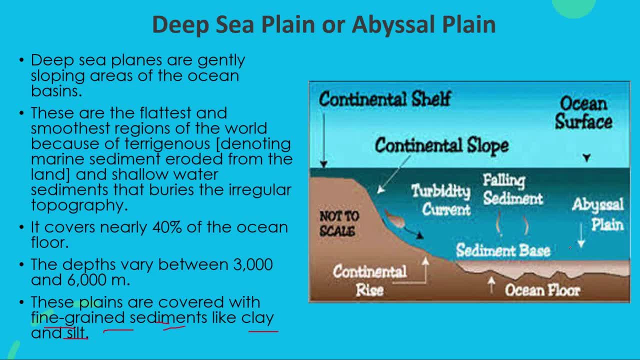 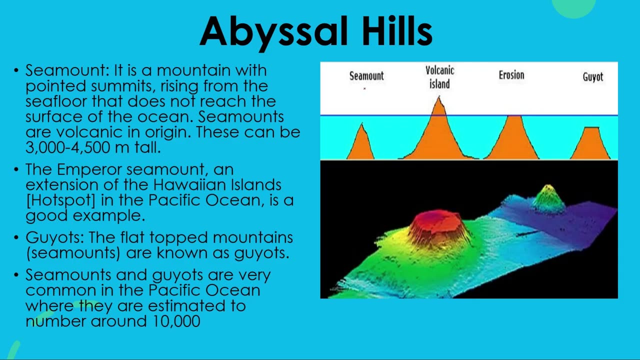 basins lies, and these are the flattest and smoothest regions of the world. okay, we have to take care of this thing. then we talk about abyssal hills. okay, if there is an abyssal plane, now, abyssal hills are coming. so, abyssal hills, there are four types of it. you will see here. 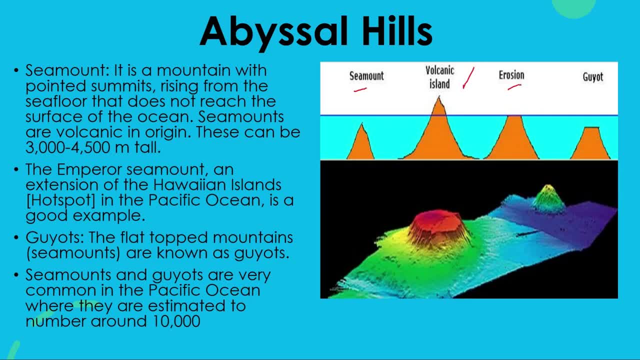 sea mount, volcanic island erosion, geodes right. firstly, seamount. seamount is a mountain with the pointed summits rising from the sea floor that does not reach the surface of the ocean. take volcanic: in origin can be from uh can. height can be varied from 3000 to 4500 meters. 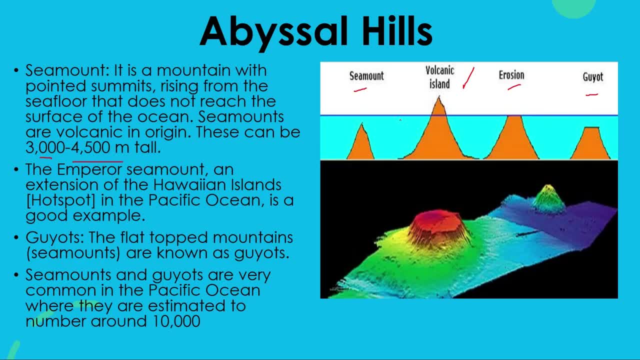 now see simple logic and classification is visible here without any problem. from seamount: okay, they are not going to reach the ocean floor. their peak will be high means the peak will be very sharp, along with the first thing of volcanic origin, volcanic islands are those which are emperor seamount- okay, an extension of the hawain island. 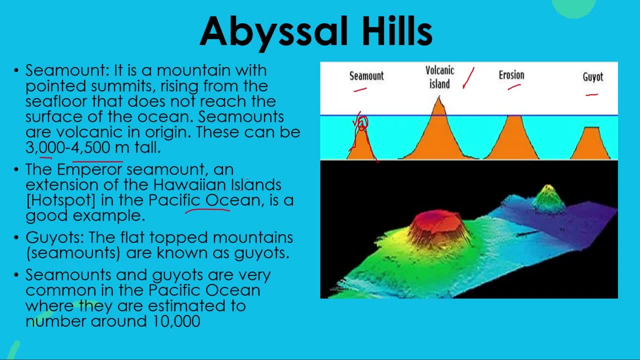 in the pacific ocean is also a good example. if you see hawain island in their map, then we can see the two are. there are two volcanic islands and the last thing that is known is that the volcanic islands are such islands, which are on the surface of the sea means they are. 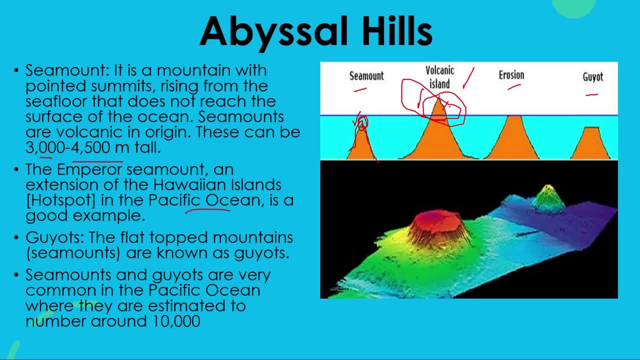 reaching such a surface above, okay. second, here are volcanic activities. volcanic region is very active. and the third is their peaks. also, volcanic peaks are very sharp. obviously they will meet, okay. so here is the hawain island. then let's talk about the gods, our gods. those left to the top of the mountains are what they are known as stars that we need. 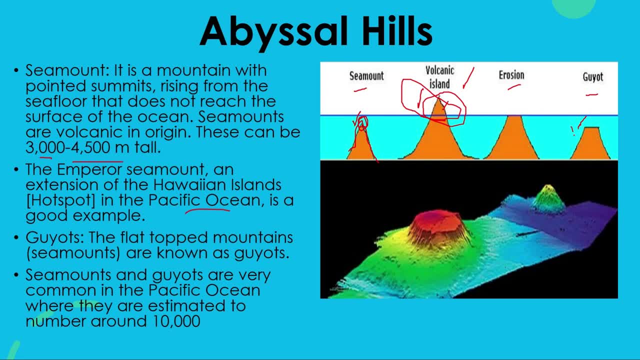 you to have. they are, there are. they are like kauravas and some will be called as saurians. there are glabras, you can see. the third one is like a small island, like seawater, the island which does not reach the height of the ocean floor. 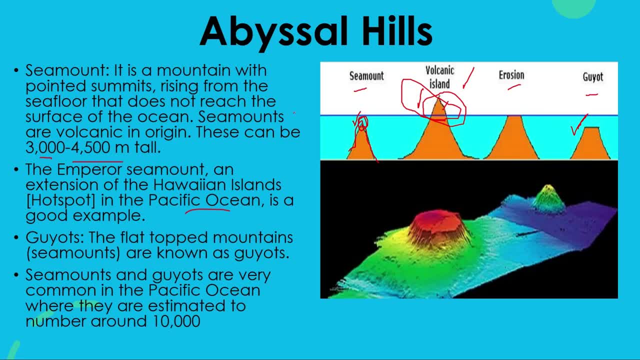 What is common between Gaiots and Seamounts? Both are not touching the ocean floor, and the difference is that the peak of Seamounts is sharp and the peak of Gaiots is not sharp. Seamounts originate from volcanic type, and this does not happen with Gaiots. 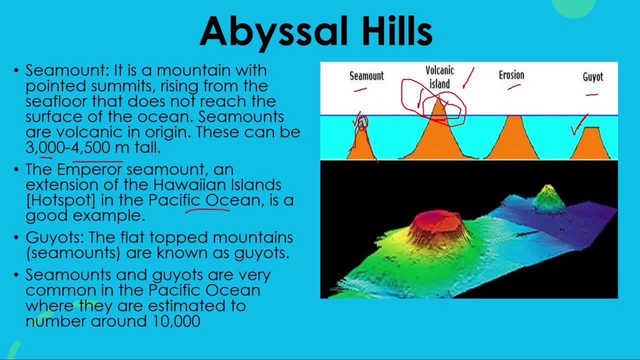 Then Seamounts and Gaiots are very common in the Pacific Ocean region, where they are estimated to be around 10,000.. If we do not look for Gaiots and Seamounts in the Pacific Ocean, or if we look at the map book, 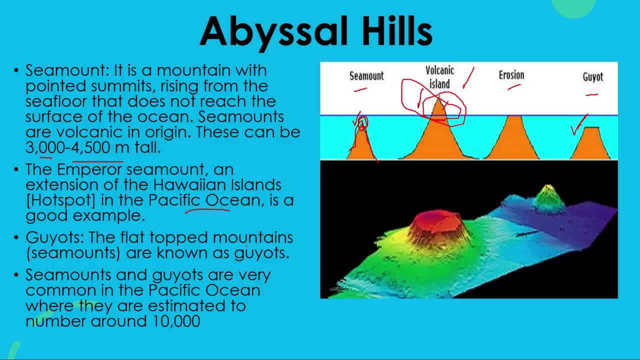 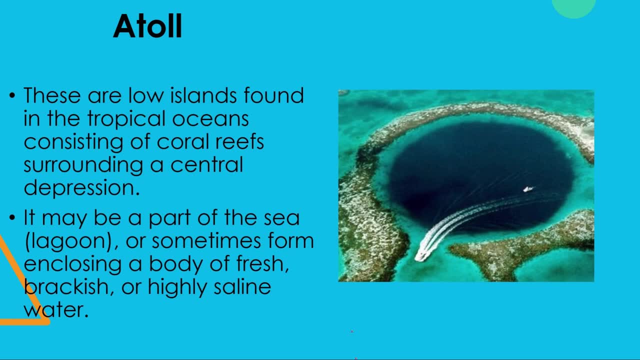 then there are numerous numbers of Seamounts and Gaiots present in the Pacific Ocean, whose approximate number is around 10,000.. Then comes the Atolls. What are the atolls? These are the low islands found in the tropical oceans, consisting of coral reefs surrounding a central depression. 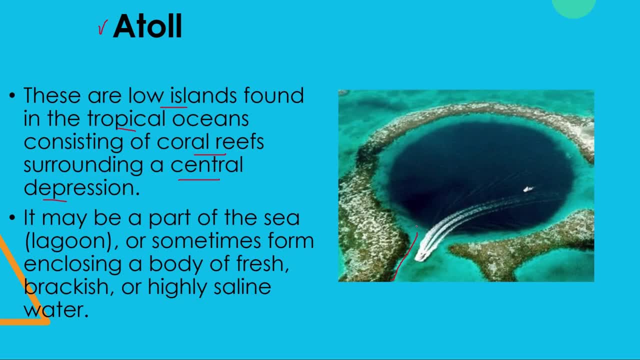 Now look at this region. You can understand that there is a depression here. This is the center region, and there is a depression here. There is something around it. This is actually our coral reefs, And the depression in the center is called our atoll. 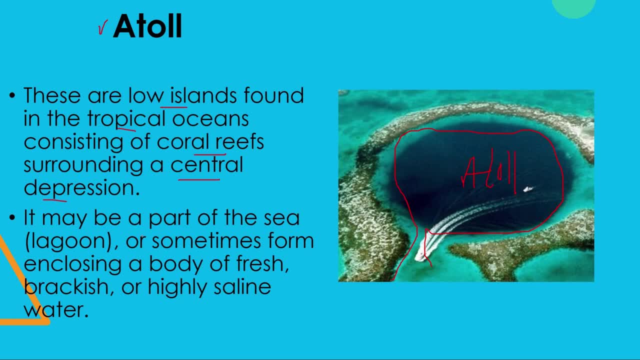 So this region is called atoll. It may be a part of the sea that is the lagoon, or sometimes forms an enclosing body of fresh, brackish and highly saline water. We have talked about water. There are three ways of salinity. 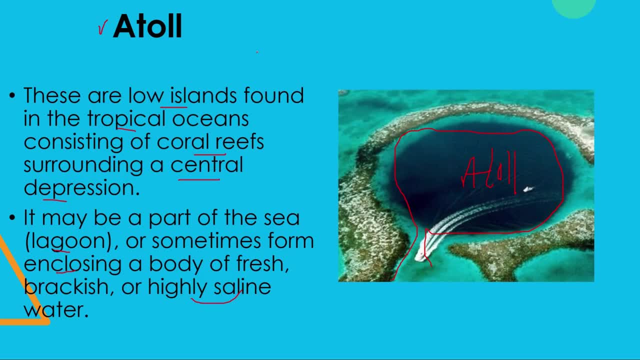 One is saline, one is brackish and one is fresh. Saline is the water whose salt content is above 35 ppd. We call it saline water. Fresh water contains zero salt And brackish water is the water whose salt content is more than the fresh water. 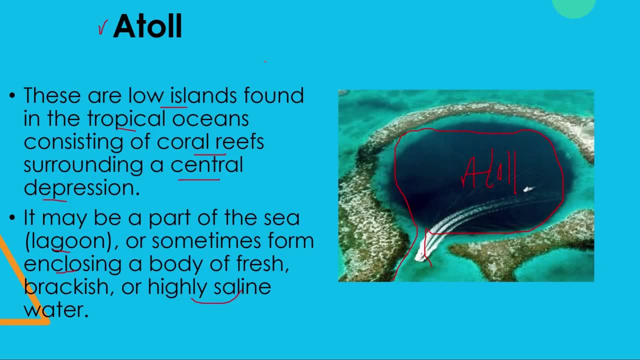 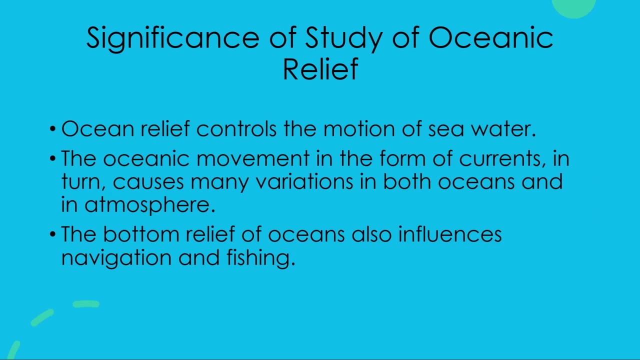 but lesser than the saline water available. So in many regions you will find a lagoon in the middle of the sea, But sometimes these are different, differing from the sea. The basis depends on the water's properties. Now the thing is that we are studying so much ocean floor. 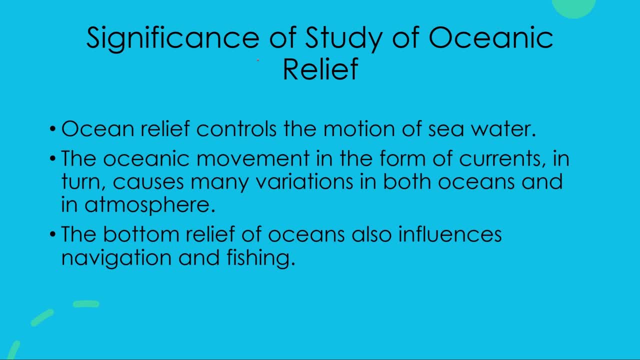 We are understanding the significance of these things. So the ocean relief controls the motion of seawater. The oceanic movement in the form of currents in turn causes many variations in both the oceans and the atmosphere, And the bottom relief of oceans also influences navigation and fishing. 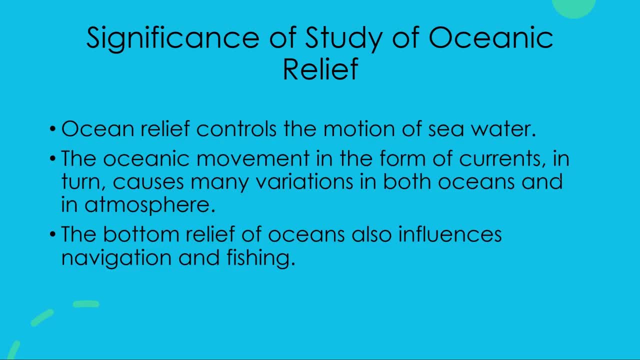 Now, if there is ocean relief, then the motion of the seawater controls and relieves the ocean. If you have a region like this, if you do a normal, practical, whenever you do that you control your ocean, you should spread a bottle of water on the flat ground around you. 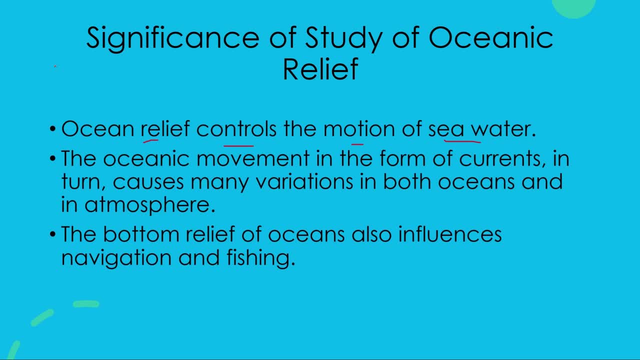 If you spread a bottle of water on it, you will see that the water moves very quickly. It moves in one direction without any problem. But if you do that, you should keep small objects in the region from where you are throwing the water. 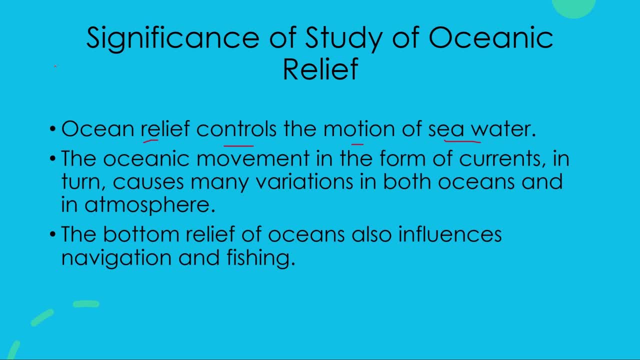 Keep any small object or anything like that, so that it is not possible to move the water in the same direction, And then you should spread the whole water. So you see that what the water does is that it changes its direction. It changes the direction. 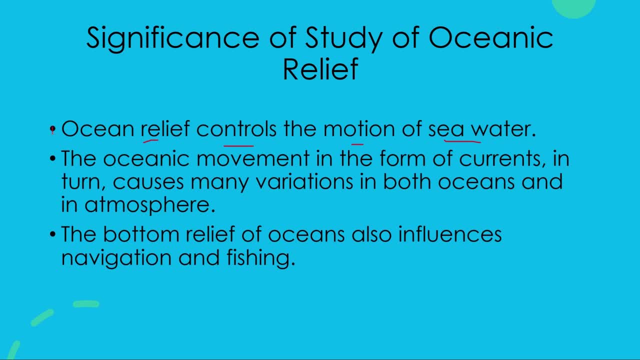 After that, what is happening here is that as soon as our ocean is relieved, our seawater will move. Secondly, the oceanic movement is in the form of currents, So we have two types of currents here. We will study the two types of ocean currents in the future. 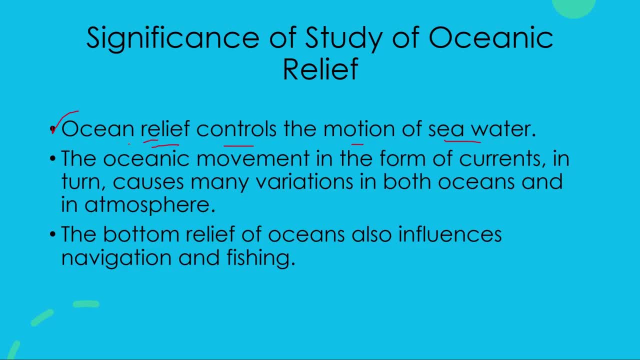 That are the cold current and the warm current. So the cold current and the warm current not only come in the ocean but also come in the atmosphere And, due to variations, such countries or such continents which are situated in the oceanic coastal regions. 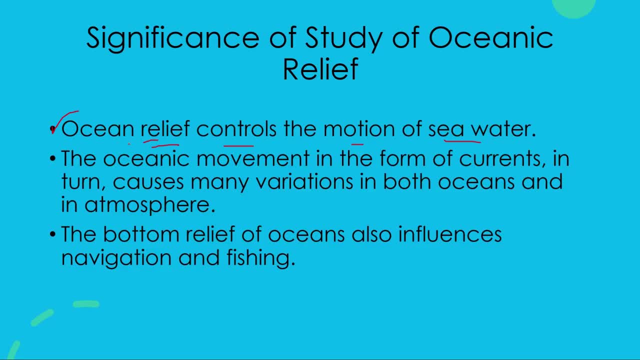 the oceanic around which a warm current or a cold current passes, a lot of things also have an effect on their country, Just because of this water movement Right, Thirdly, we are saying that the bottom relief of ocean also influences navigation and fishing.